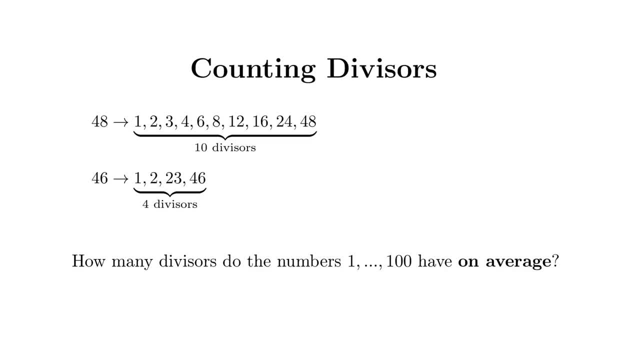 on average. Even though the task is easy to understand, coming up with a reasonable guess for the average is well tricky, and right now nothing indicates that the answer is connected to Euler's number. So the general question we will tackle is to find a formula which approximates how many factors the numbers from 1 to n have. 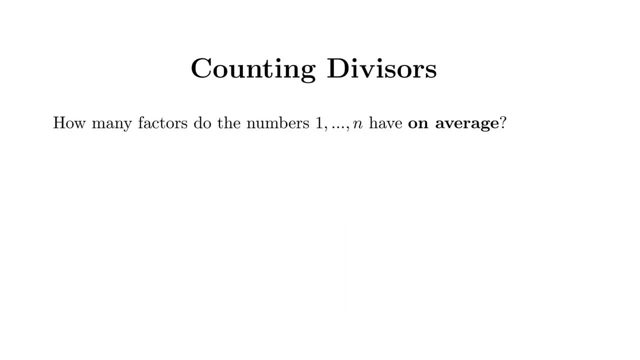 on average. I love this problem for three reasons. First, everyone knows what divisors are, making it not only a simple question to understand, but also many people have at least some sort of intuition for it. Second, it shows how very different fields in mathematics can work together In this. 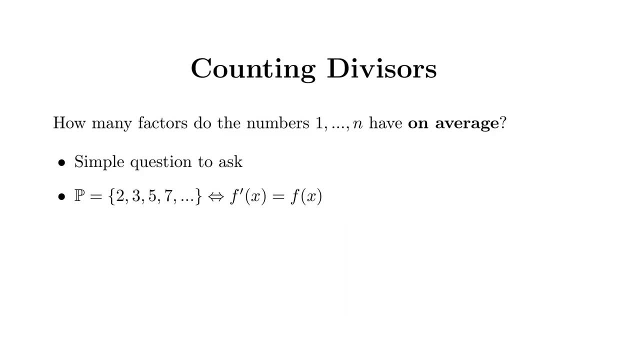 case, number theory, which often deals with studying prime numbers and analysis where, where Euler's number was born Last, every single step of the solution can be visualized easily, therefore avoiding dry calculations and making it more accessible. That being said, let's dive right in. 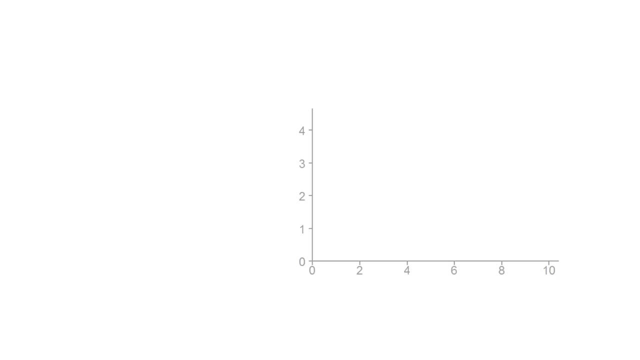 So we can count for each integer its factors. As an example, for every number from 1 to 10, the number of factors is listed. Note: prime numbers are easy to spot as they only have two factors, namely 1 and themselves. 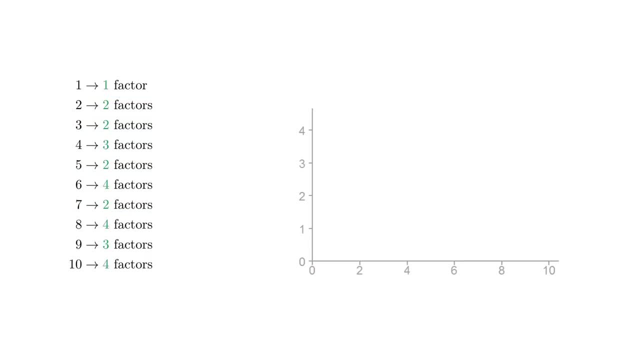 As our goal is to understand how frequent divisors are, let's start by getting a feeling for how common factors are and visualize this number of factors. For instance, 6 has 4 factors. we get the point. Doing this for every number, we end up with this wonderful picture. 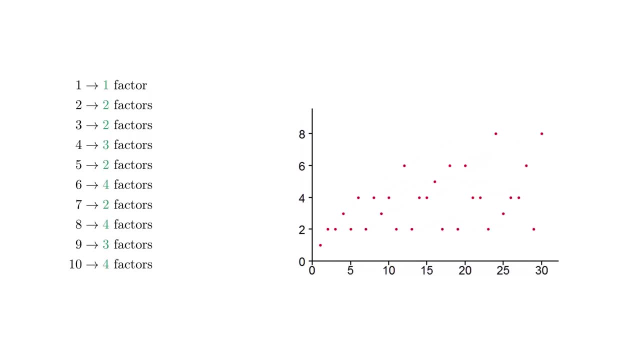 When zooming out, the pure chaos behind the number of factors becomes apparent, and this chaos alone certainly cannot be captured by a simple formula. So let's address our main question of how many divisors a number has on average. So as a start, say we want to find the average number of factors. 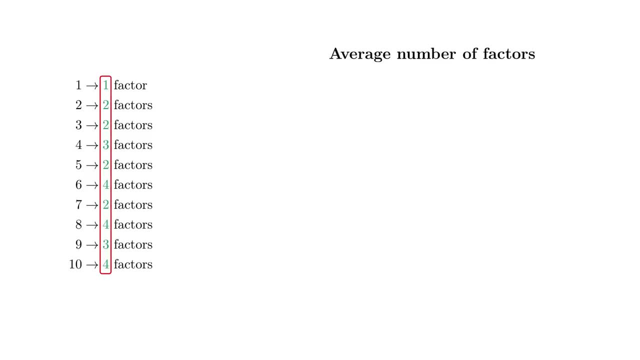 that numbers from 1 to 10 have. Well, we get the average by computing the sum of the number of factors and dividing it by 10, equalling 27 over 10, or 2.7.. Hence, random number from 1 to 10 has an expected number of factors of 2.7.. Doing, 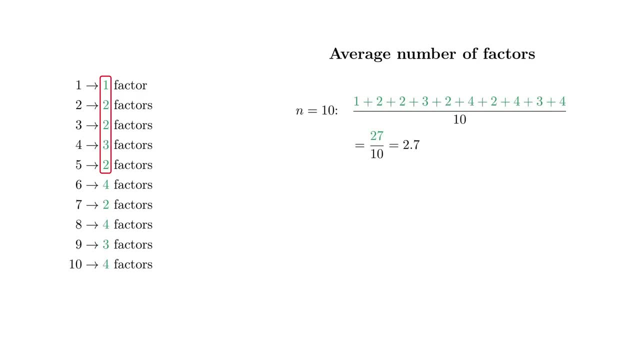 the same for the first five numbers. we end up with 10 over 5 or 2.. Again, as we want to understand how these averages grow, let's visualize them. We have the point 10,, 2.7,, the point 5,, 2 and we end up with this rather smooth growth which? 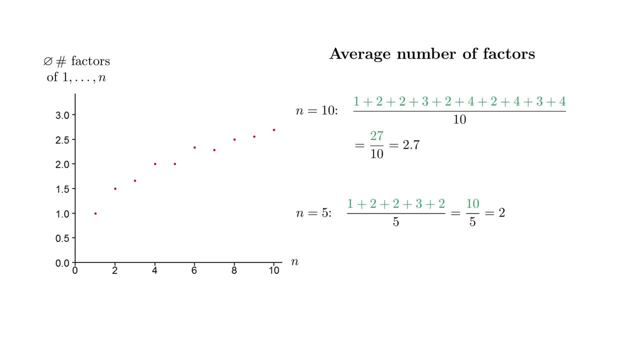 makes sense, as taking averages decreases variance. Simply to make the graph look prettier, I will connect these dots and then zoom out once again. Well, wow, suddenly the chaos from before disappears completely and we end up with this almost perfectly smooth curve representing the average number of. 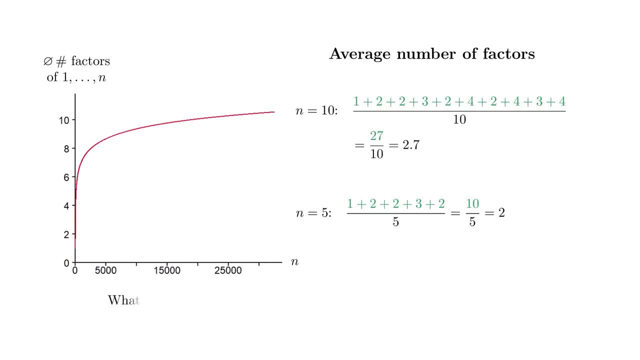 divisors. If you're anything like me, you just have to know what this curve is and why it appears. To unravel this mystery, we have to take a step back and come back. We end up with a new way of counting divisors from 1 to n in a systematic way. Take for 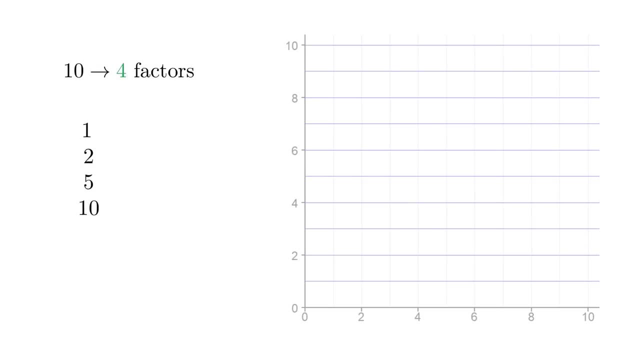 instance 10 and its four divisors, Sort of. the reason why they are factors of 10 is that each of them has a counterpart, such that their product equals 10.. Put differently, there are exactly four ways to write 10 as the product of two. 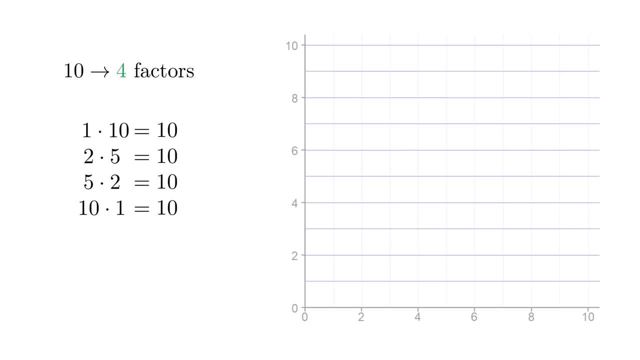 natural numbers. As we now deal with pairs of numbers, we can start plotting them in the xy-plane, So as 1 times 10 equals 10, we get the point with x-coordinate 1 and y-coordinate 10, and similar for the other three points. 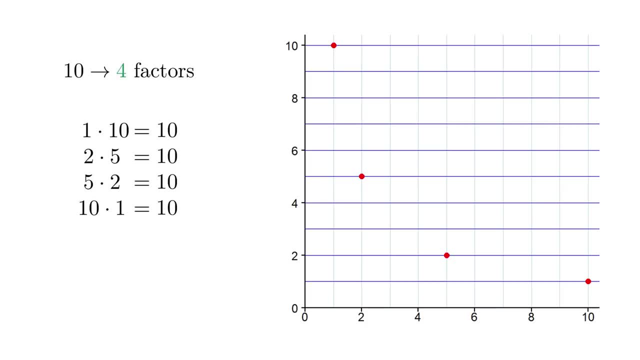 Notice we are visualizing whole number solutions of x times y equals 10.. As this equation can be rewritten as y equals 10 over x, we can also plot the graph of this function, which happens to be a hyperbola, going through our four points. 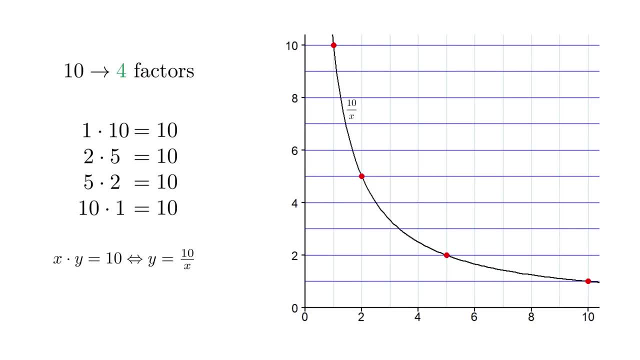 Importantly, these are precisely the integer lattice points of the hyperbola, as these correspond to pairs of numbers who are the final number and whose product is 10.. If we now continue plotting the hyperbola- 9 over X- we see that there are precisely three points on its graph of. 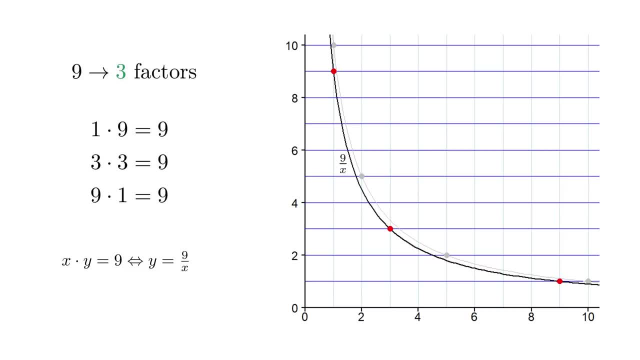 integer coordinates, namely 1, 9,, 3, 3 and 9,. 1 corresponding to the three divisors of 9, namely 1, 3 and 9.. For 8 over X, the hyperbola goes through four. 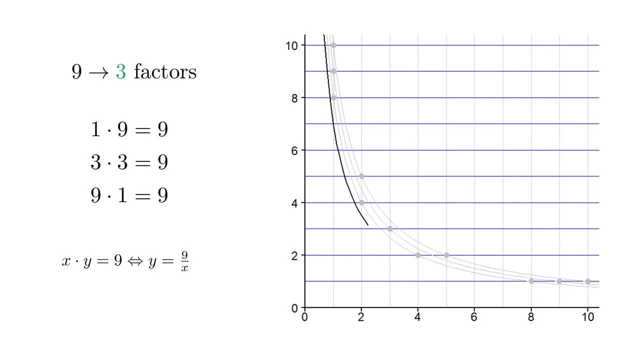 points corresponding to the four factors of 8: 1, 2, 4 and 8 itself. Continuing this procedure, we end up with every single whole-numbered point as a number that is on and below the original curve, corresponding to every factor of every number, from 1 to 10.. 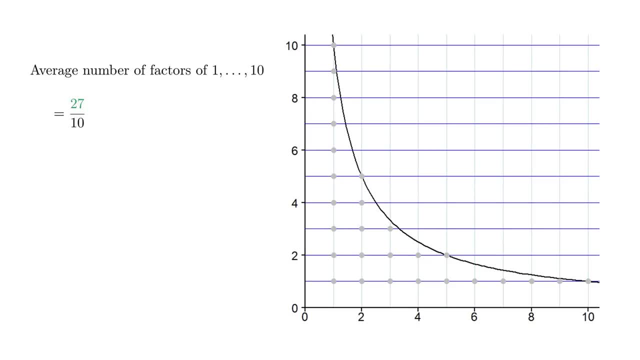 Here one should point out that we already computed the average number of divisors of a number smaller than or equal to 10, which was 27 divided by 10, where the 27 counted all the divisors of all numbers, from 1 to 10.. 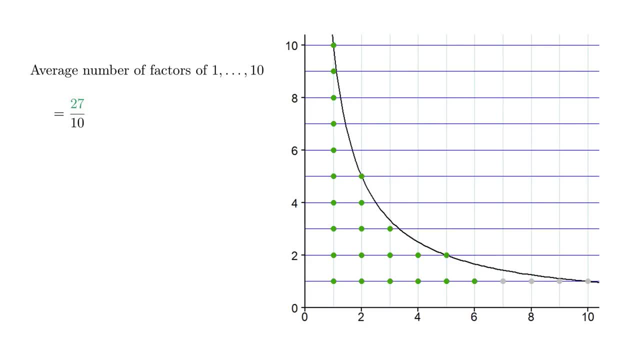 As we are now precisely visualizing those divisors, it makes sense that they are precisely 27 points below the original graph. This encourages us to ask a new question: How many integer points are below a given hyperbola? So is there a formula describing this quantity? 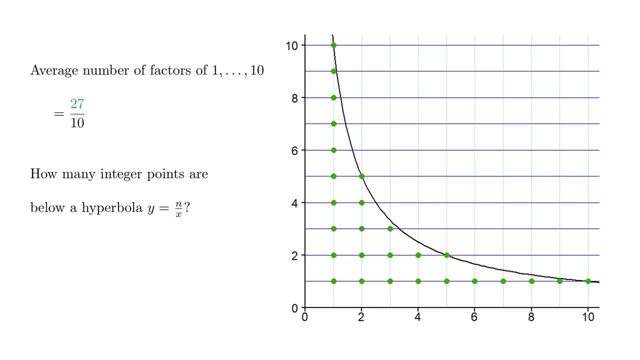 At first. there is not really a clear way to count such points, as a more common question is to ask about the area below a given graph. With this in mind, let's squareify the points. Let's add for every point, a square with side length 1,. 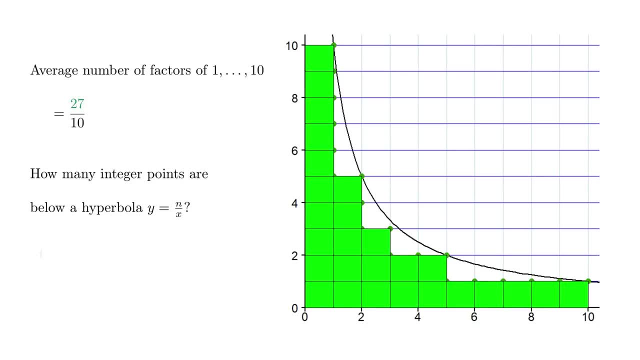 which is directly below and to the left of the point. As all these squares have area 1, the total area they have simply equals the number of points. Unfortunately, this area still isn't easy to compute, So let's make two simplifications. 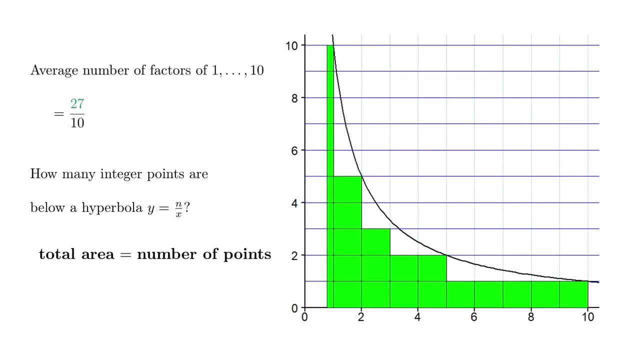 First, we get rid of the first column and second, we add this extra strip on top Immediately. we thereby change the total area. However, doing the same for, say, the first 30 numbers, we see that the error created has only a small effect. 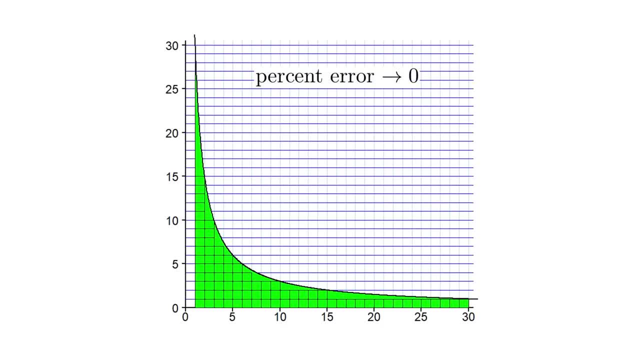 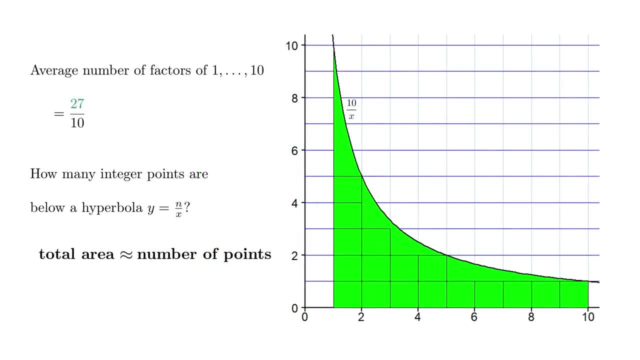 In other words, in the long run, this simplification does not change the result, as the percent error tends to zero Going back. the number of factors of a number smaller than or equal to 10 is now approximated perfectly by the area below the curve 10 over x. 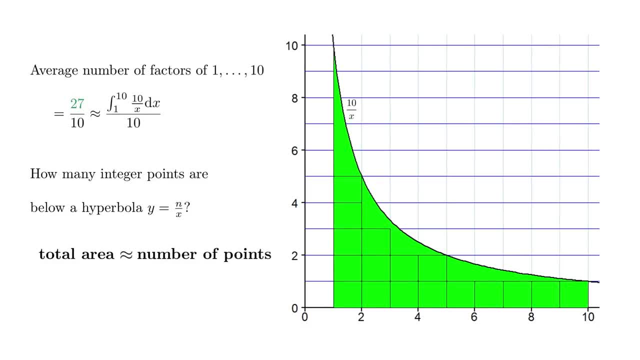 from x equals 1 to 10.. And well, this can be computed by this example. The number of factors of a number smaller than or equal to 10 is now an integral. so suddenly we have to use calculus to answer the simple question. 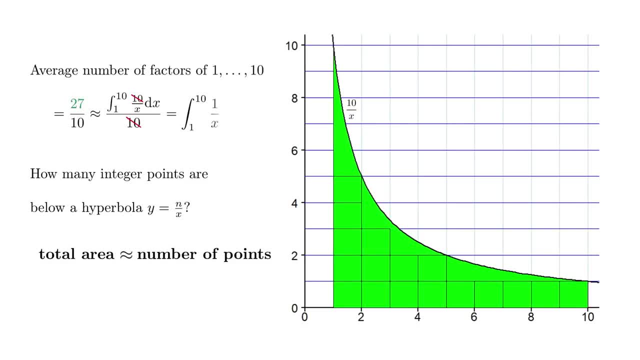 of how many factors a number has on average. Cancelling the tens, we end up with the integral from 1 to 10, of 1 over x, dx. You might guess correctly that by replacing 10 with any whole number, n in general. 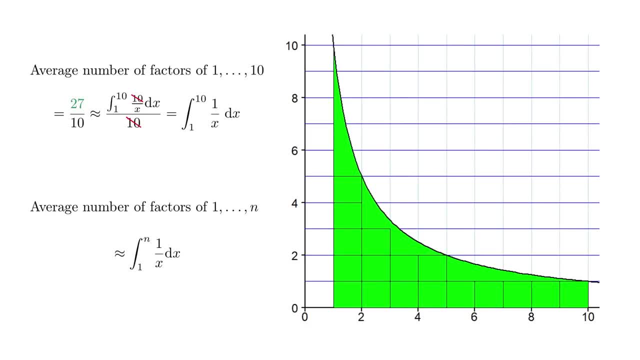 we arrive at the result that the number between 1 and n has about this many factors again, where the percent error goes to zero. So how can this integral be computed? Well, we have to look for a function whose derivative equals 1 over x. 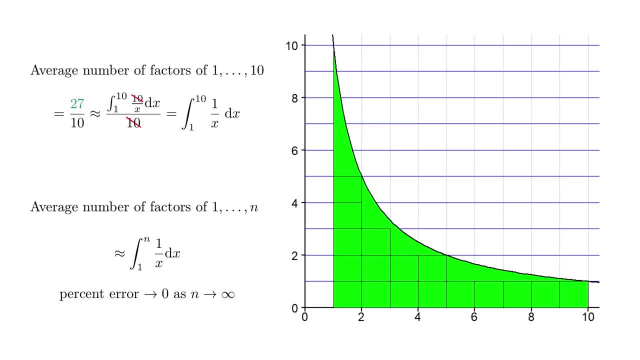 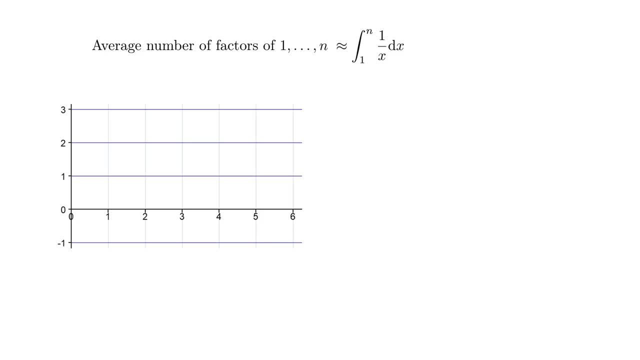 It's now time to introduce Euler's number as the star of this video. So a number below n has, on average, this many divisors. In order to compute the integral, we have to find the function whose slope at any point x equals 1 over x. 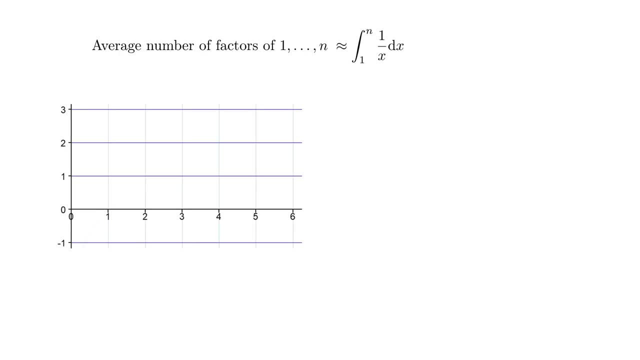 The mysterious function that we are looking for has to look something like this. It has to have: at x equals 1, a slope of 1,. at x equals 2, a slope of 1. half. at x equals 3, a slope of 1. third, 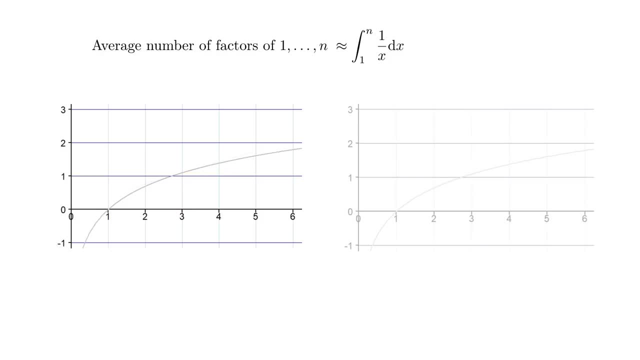 and so on. We get something that looks much like the graph of e to the x we had in the beginning, but somehow flipped More precisely, the x- and y-axis seem to have changed place. Hence everything got mirrored along the 45-degree axis. 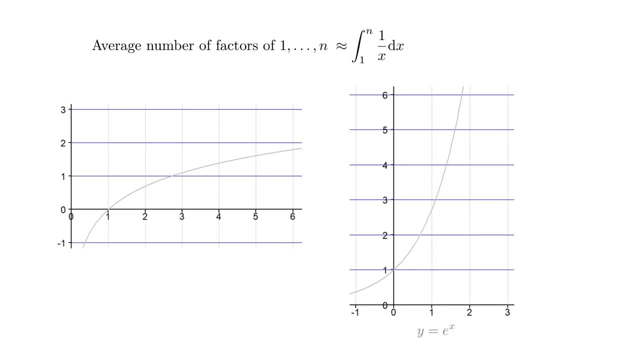 So maybe we shouldn't focus on the equation e to the x equals y, but instead e to the y equals x. therefore, switching x and y, This means that y equals the logarithm of x, or more precisely, the natural logarithm of x. 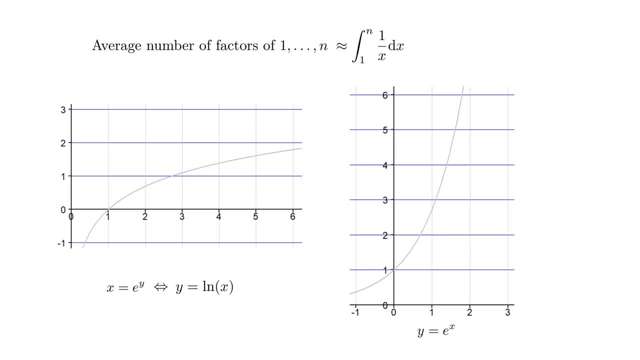 as it has Euler's number as basis. Last, we need to check that the slope of log x indeed equals 1 over x. As an example, why should the slope of the tangent at x equals 2, be 1 half? Well, first, 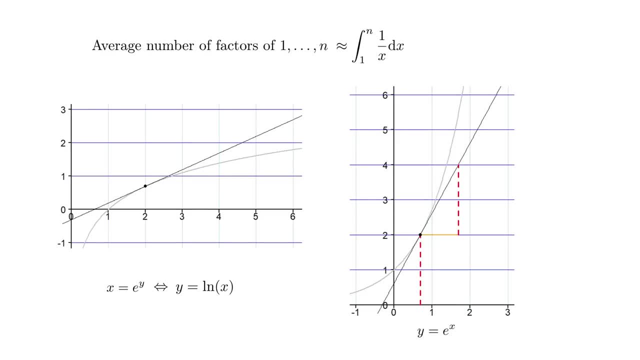 the two dotted lines of the exponential function have the same length, in this case 2,. as we saw in the beginning, This translates to these two dotted lines of the logarithm having equal lengths. If we now rearrange the sides and shrink the triangle by a factor of 2,.